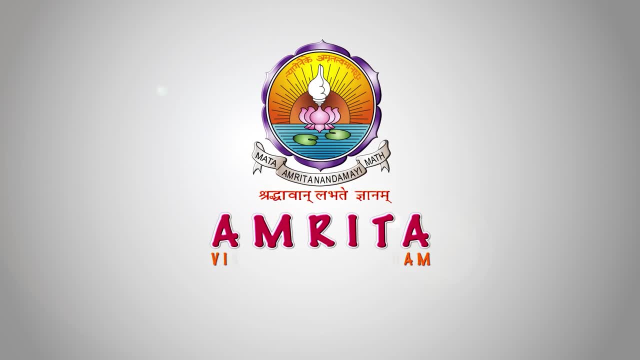 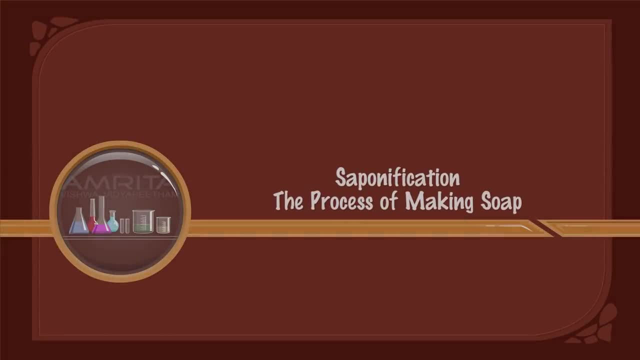 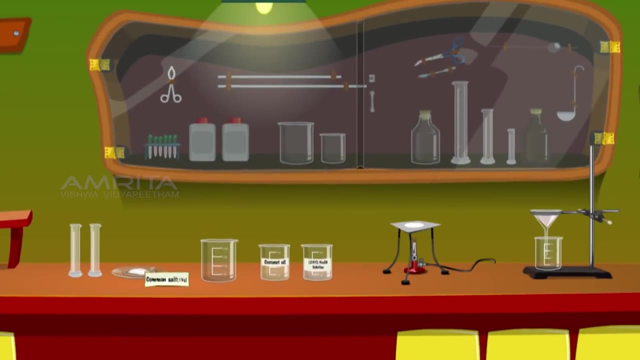 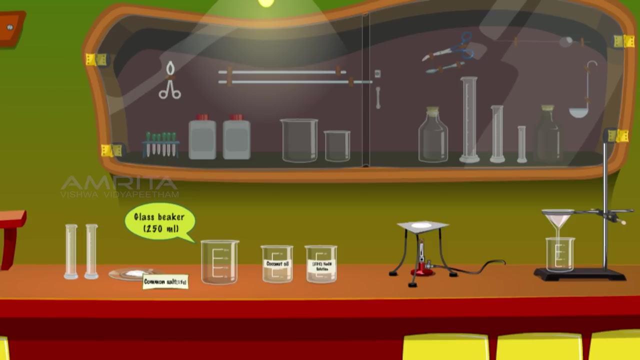 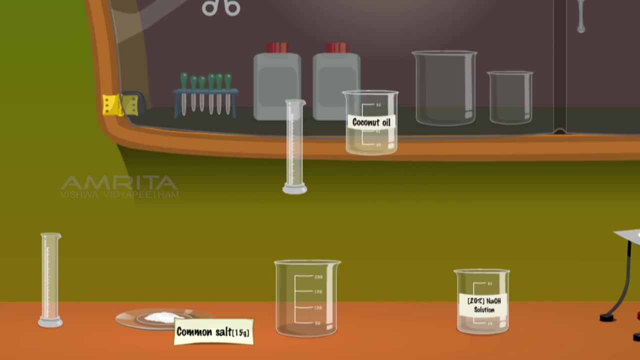 We require measuring cylinders, common salt: glass beakers. coconut oil, 20% NaOH. coconut solution. Bunsen burner funnel. Measure 25 ml coconut oil into a measuring cylinder. Pour the oil into a glass beaker, Take another measuring cylinder and measure. 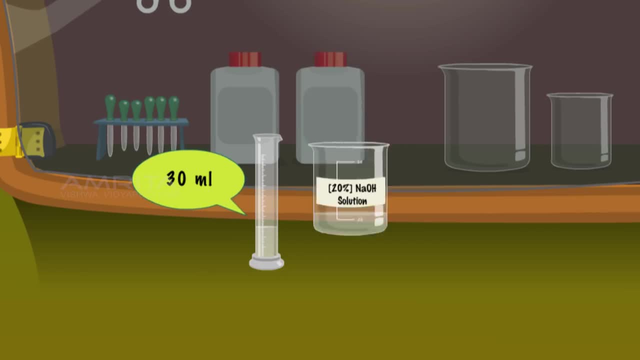 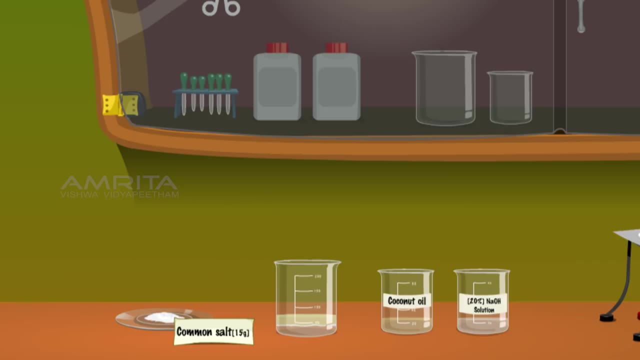 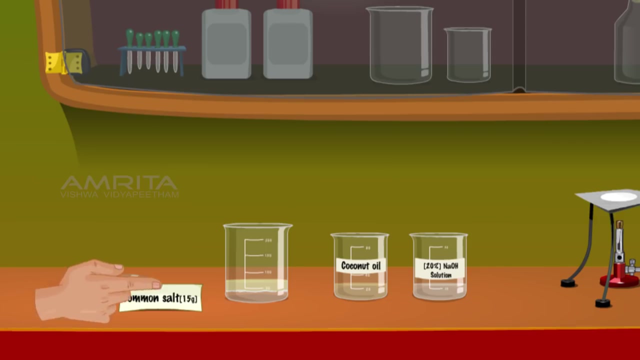 30 ml 20% NaOH solution into it. Pour it into the beaker containing coconut oil. Stir the mixture vigorously Using a glass rod. touch the beaker from outside. It will be observed that the beaker is warm. This is due to the exothermic reaction between vegetable oil, ie coconut oil, and sodium. 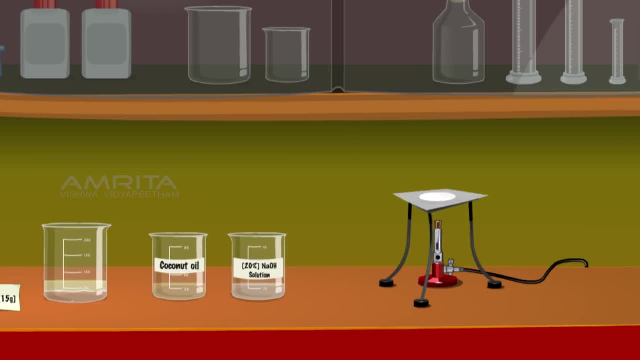 hydroxide solution. Place the beaker on a Bunsen burner and heat it until the mixture becomes a whitish paste. The mixture is made up of sodium hydroxide solution. Heat the mixture for about 10 minutes To make the mixture coagulate. take a piece of cloth and place it on a sheet of foil. 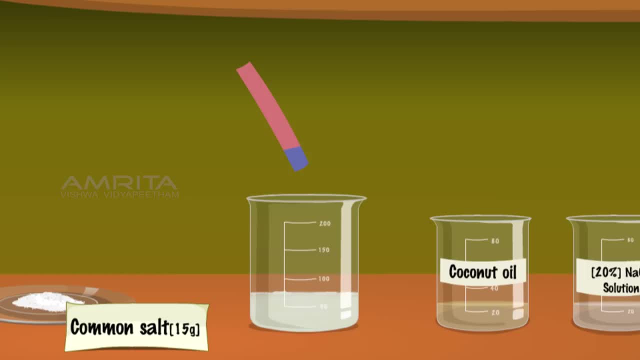 Remove the beaker from the flame and allow it to cool. Dip a red litmus paper in the suspension formed. When dipped in the suspension, red litmus paper changes to blue colour. This shows that the soap solution is basic in nature. Dip a blue litmus paper in the suspension. The colour of blue litmus paper remains the 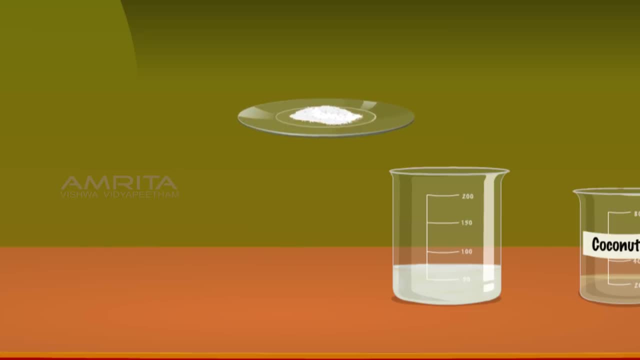 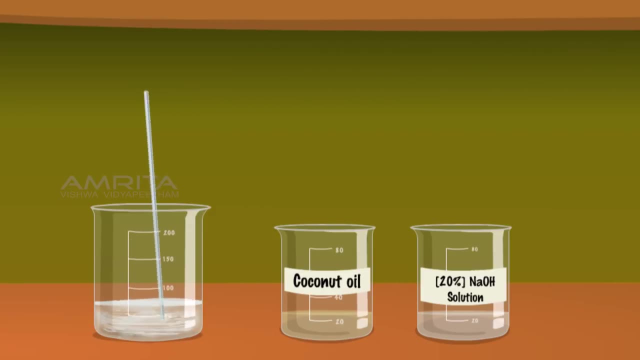 same. This shows that soap suspension is not acidic in nature. The mixture is ready for use. acidic in nature. Add 15 grams of common salt into the suspension. Stir it well with a glass rod. It is observed that the soap is precipitated out as a solid.